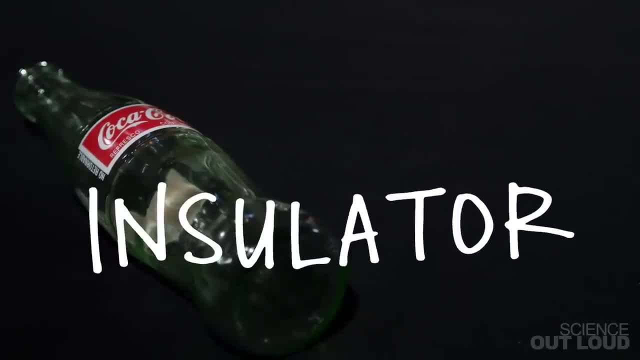 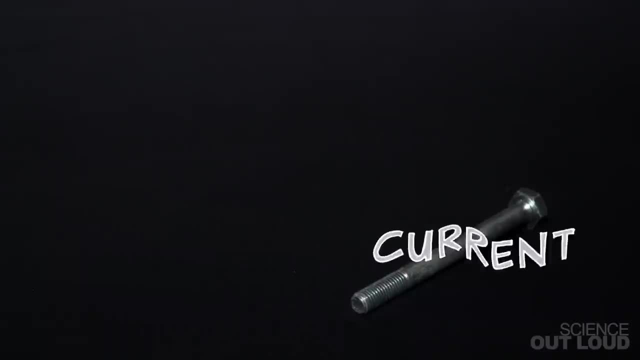 so current can't flow And it's an insulator like this. glass Metals have no gap at all. Electrons can move to the higher energy levels with no problem. Current can flow. Semiconductors fall somewhere in the middle. They have a medium-sized band gap, So technically, 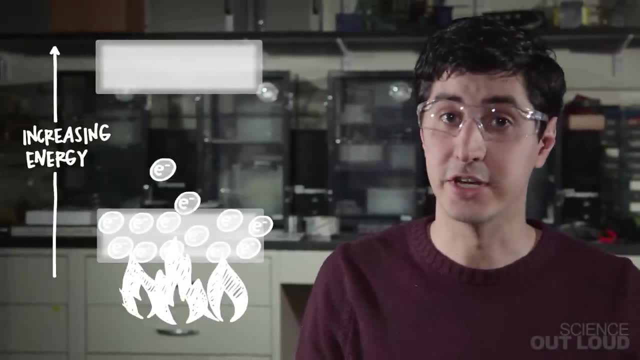 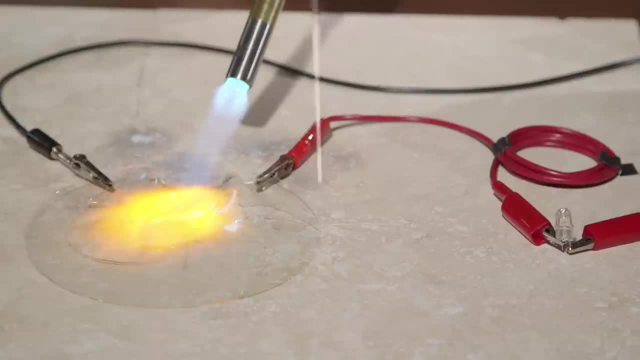 I can make this glass conduct electricity if I added enough energy through heat to push the electrons into a higher band. But that amount of heat would either melt or break the glass before it actually conducts. This is true of most insulators. The amount of energy needed to 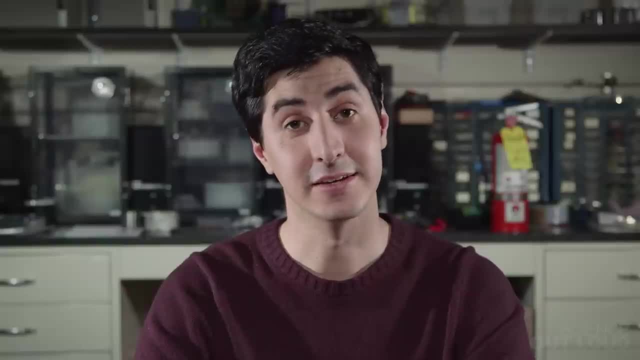 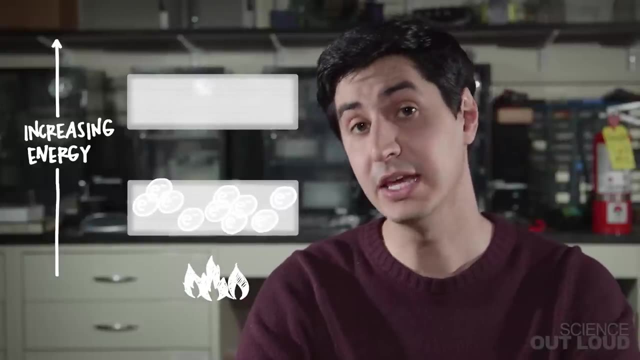 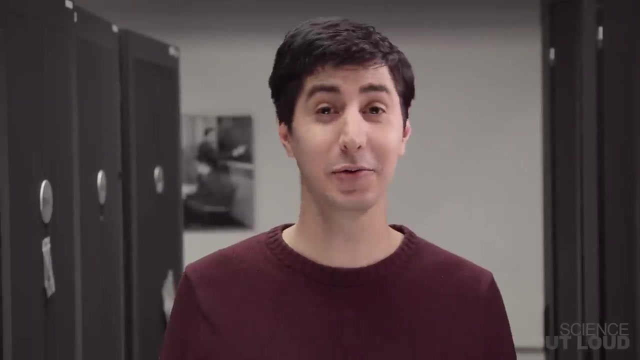 make them conduct is just too high. But in a semiconductor the band gap is small enough that electrons can jump into the higher energy band so that current can flow. The amount of heat we apply determines how many electrons jump into the higher band and how much current flows. And heat isn't the only way to change the 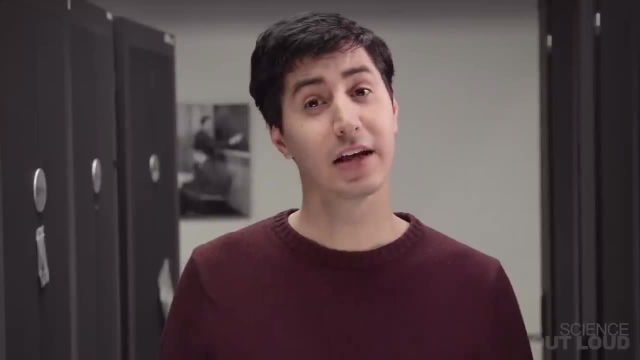 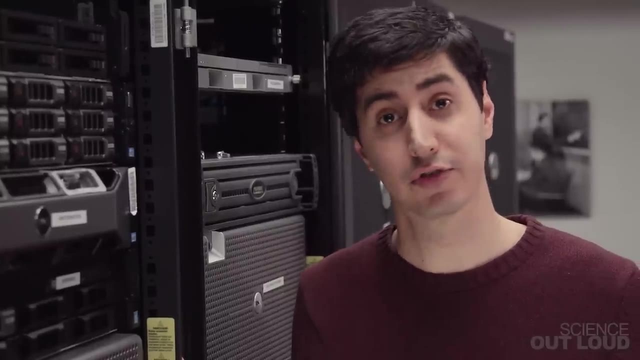 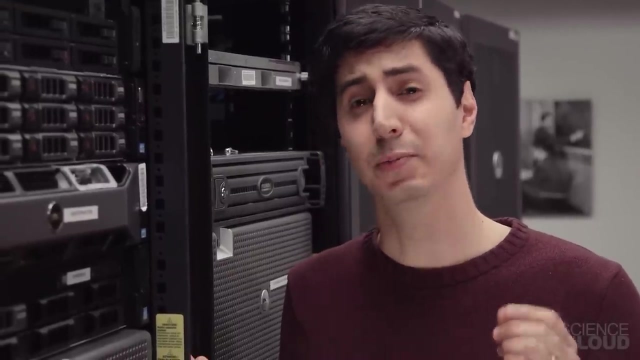 conductivity in a semiconductor, We can also use light electric currents and, in a computer, electric fields. As I've said, computers are made up of semiconductor switches, called transistors, that switch between conducting and insulating. Computers use electric fields because heat is slow and would burn too much energy. 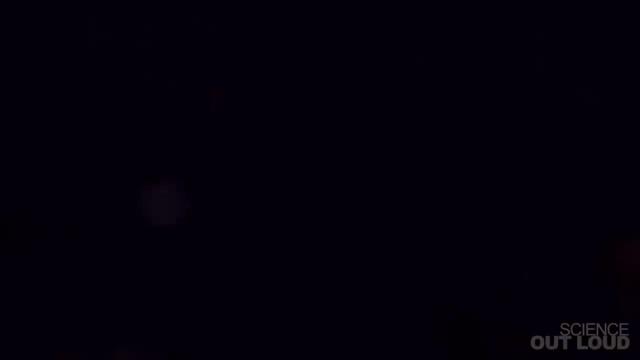 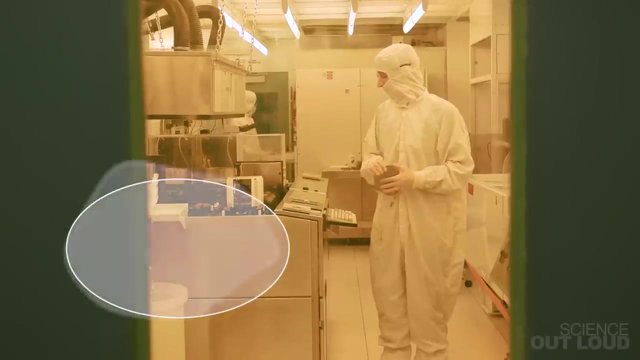 We can turn this wafer into a computer chip by printing a circuit of transistors on it using a process called photolithography. Here in the photo room, we cover the wafer with a light-sensitive material and expose it to light that we shine through a patterned mass. 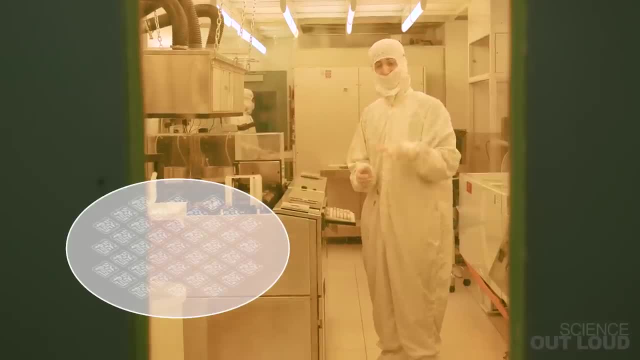 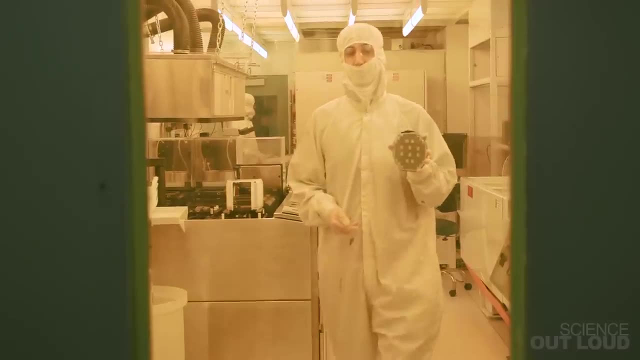 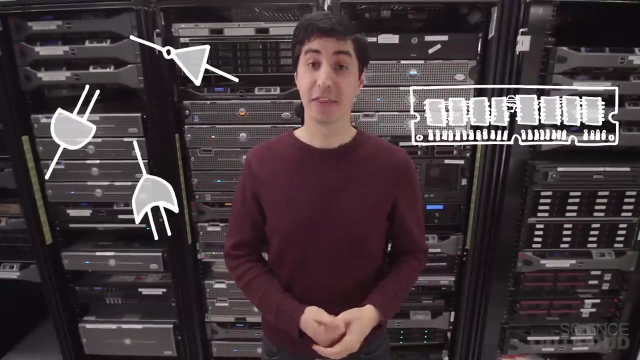 Then we develop the wafer, like film and photography, which leaves behind a pattern that becomes the circuit. Photolithography at once lets you make circuits that are smaller and cheaper than if you built them from individual parts. Transistors make up the logic elements, the memory components and the communication modules. 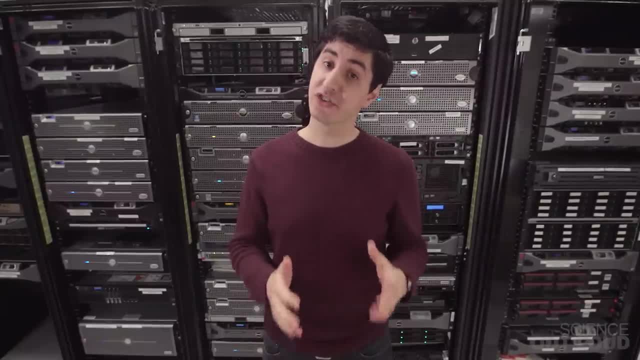 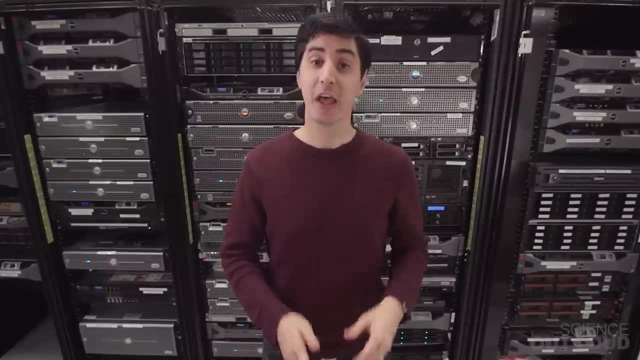 that let computers talk to each other. With semiconductors you can cheaply add transistors to almost any device you can think of, from spaceships to servers to maybe even your toaster. Semiconductors have enabled the technological revolution: the internet, the computer and